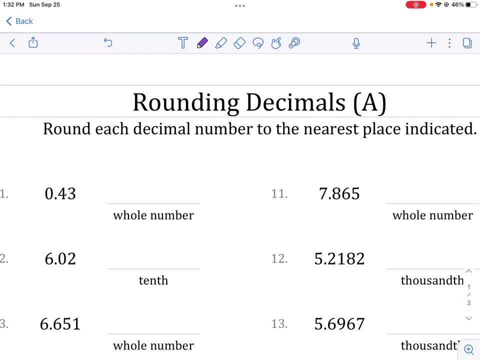 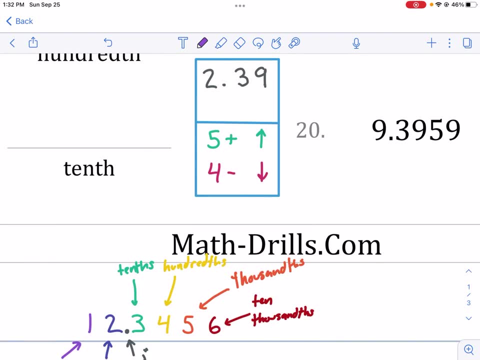 Hi, this is Mr West and today we are doing a rounding decimals worksheet from mathdrillscom. Make sure to check out the link in the description below for math drills types worksheets. They have tons of great content there and I also have playlists for their worksheets, So make sure. 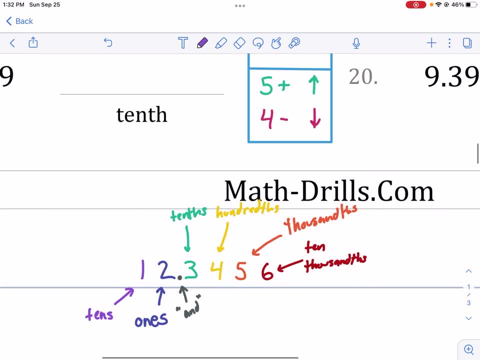 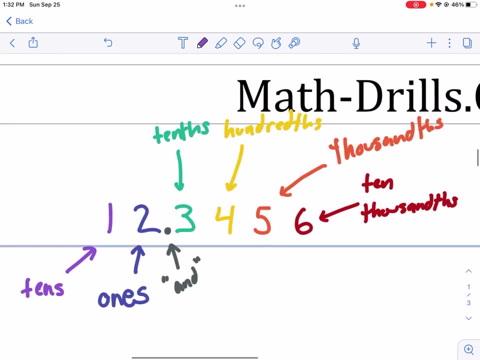 to check them out. They have lots of great resources, like I said, and I make tutorial videos for them. So this particular video is on rounding, And the first thing we need to know about rounding is how to identify all the places. If you want to pause the screen, this is a great 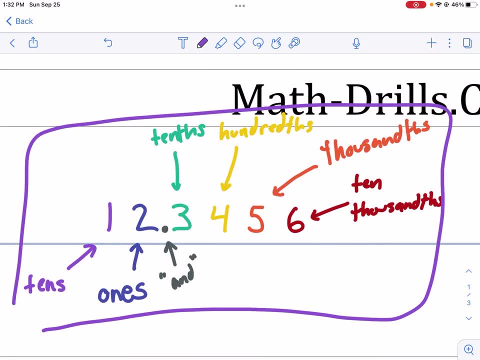 kind of start. This would be great for notes if you want to see. what do we call these different place values? So the first thing you'll know is we have this ones place. Okay, the ones place is before the decimal place. There's the decimal, The ones place is kind of like the halfway point. 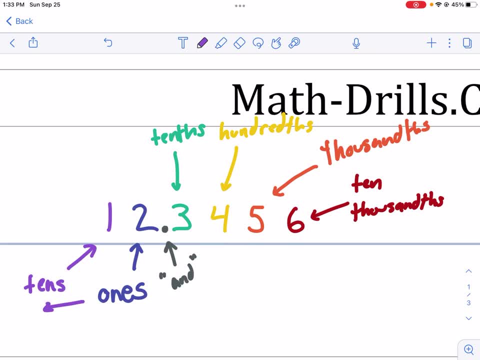 And let me kind of describe what that means. So to the left of this point we have the tens place, And then of course we'd have the hundreds place. that would be 312, that number right there, Okay, so you already knew that, But to the right of it. 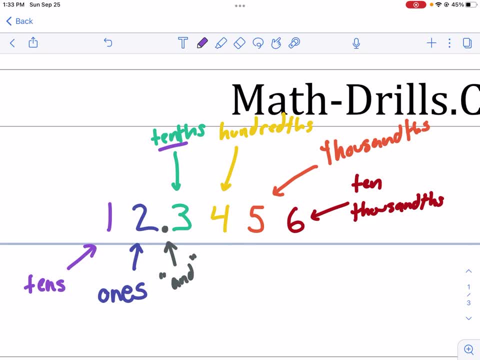 you'll know that it's the tens place, And then of course, we'd have the hundreds place. That would be 312, that number right there. Okay, so you already knew that. But to the right of it you'll notice that there's no ones place. It starts with the tens place. Okay, so we have tens to the. 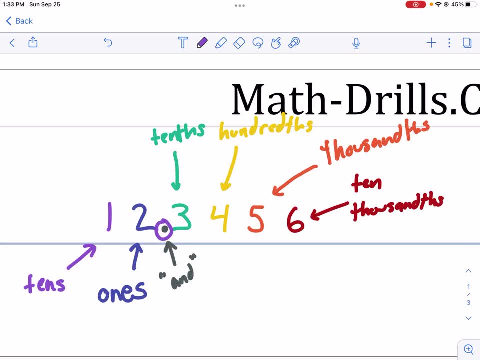 left of the ones place And then to the right of the decimal, there's the decimal, we have the tens place. Notice how all these have THS at the end of it. Okay, so how does it go? It goes tens place, hundreds place, thousands place and then 10,000 place. Now quick little summary of how do 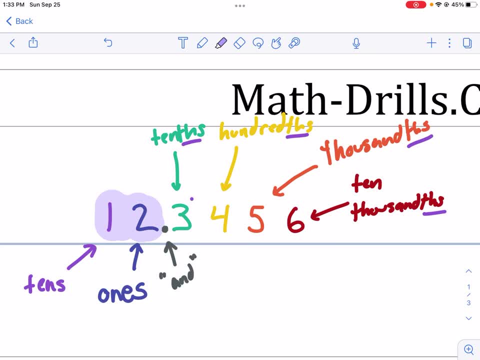 we read numbers. you first say the number to the left of the decimal, So in this case it would be 12.. Then you say: and okay, so 12.. And then you read this number as if it were by itself to the right. 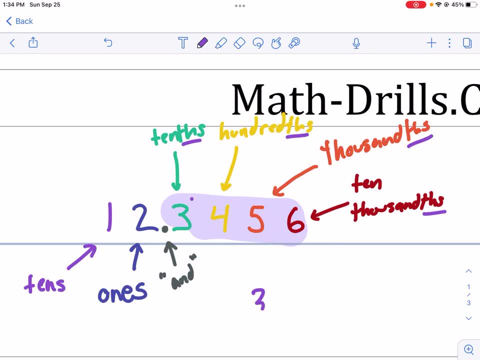 of the decimal. So you look at the number by itself And this is 3456.. Imagine if that's by itself. Okay, so we would say 3456.. And then you give it the label. the labels the last digit. So 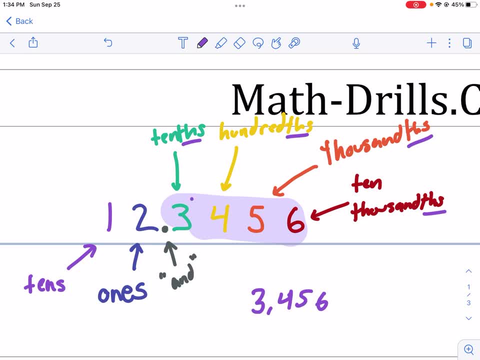 that's 10,000.. The last numbers of 10,000.. So you would say 3456, 10,000.. In total, you would say 12 and 3456 10,000.. And that's how you say it. So now that we know the places, or, if you want, 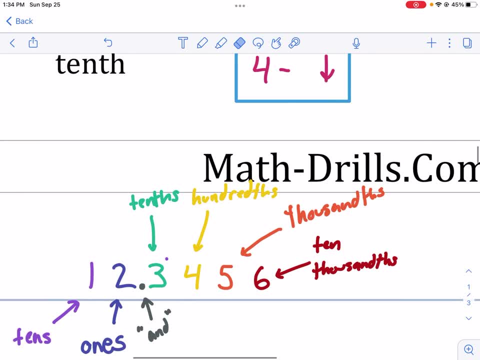 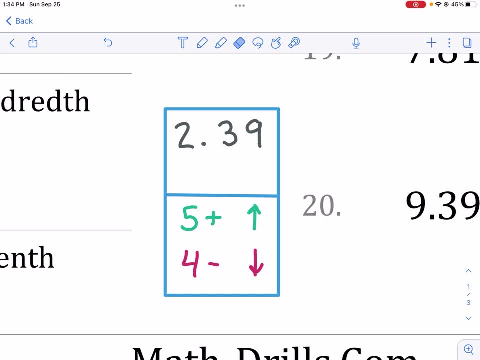 go back and rewind and get an understanding of those places. Let's apply: how do we round? Let's take this number, 2.39, or two and 39 hundredths. Let's say we wanted to round this number to the nearest tens place. So there's the tens place. How do we do that? Well, we first. 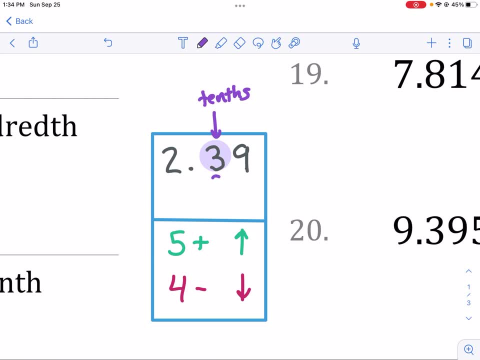 it's right there, Okay. so if you didn't know where it was, we've identified it. there's the tens place. The next thing we do is we look to the number to the right of the tens place. So the number to the right is a nine. Okay now, this nine is important because it will tell it, tell us what. 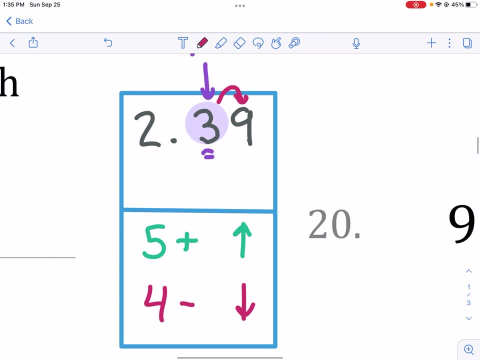 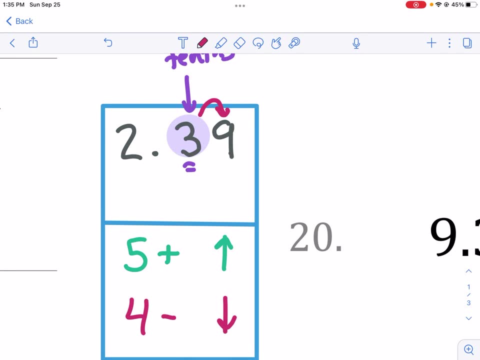 to do with this tens place. Since it's a nine, we're going to round up. That's what this little chart tells us. we're going to round up. So we're going to take this three, the tens place, and we're going to change it and round it up. 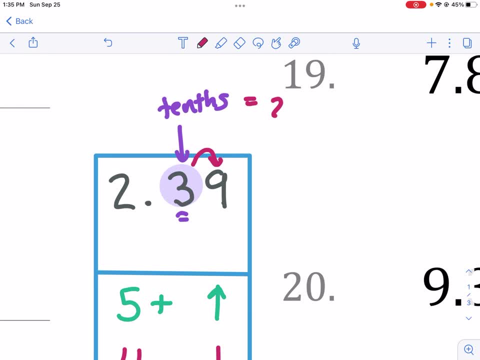 So if you're going to round to the tens place, it would become two point, instead of writing the three rounds up, because the nine is big and it rounds it closer to 2.4.. And that's how we round. Okay, because the reason why we change it to the four instead of leaving it at the three is because 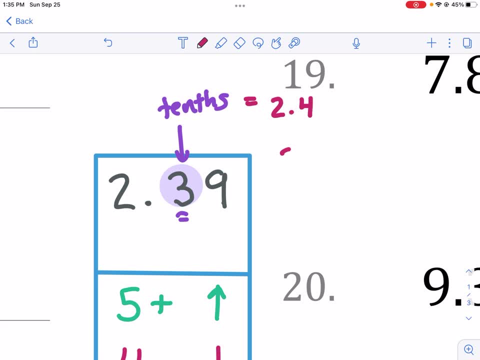 the nine gets us closer to 2.4 than it would otherwise be to 2.3.. Imagine if we have, like, a decimal line here. whoops didn't mean to do that. We have a decimal place here And we have. 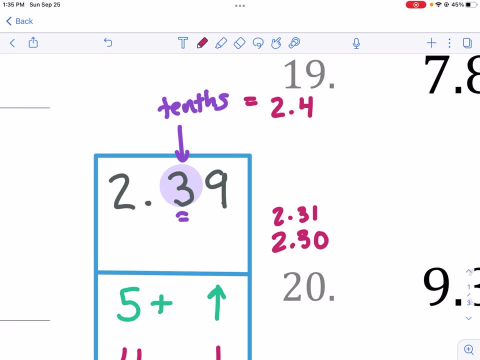 these different decimals: 2.31.. Technically, 2.3 is 2.30.. But 2.39 is clearly closer to 2.4 than it is to 2.3.. Okay, so that's why we round up. So let me erase this. we don't need any more of that. 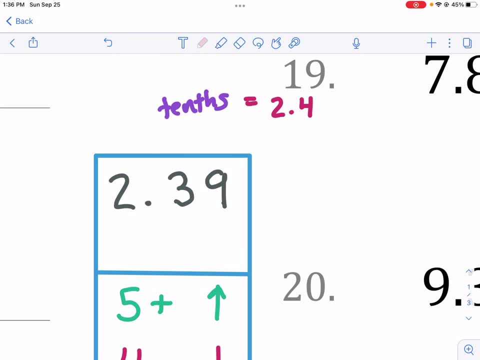 we're going to erase that. And now let's round to a different number. Let's say we wanted to round to the nearest whole number. Okay, whole number is another name for the ones place. So we need to identify the whole number or the ones place, And that is there. 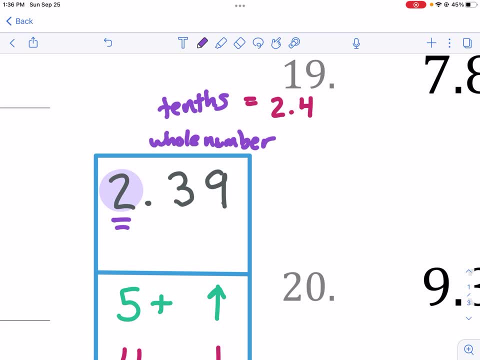 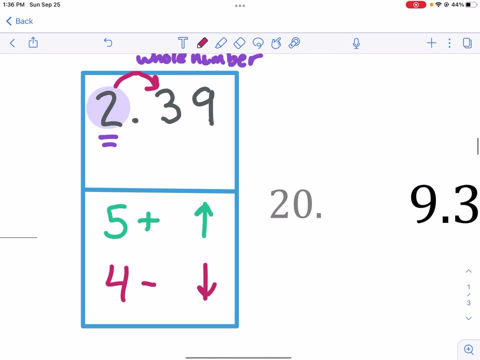 Okay, for emphasis. I'm underlining it also in case you don't have a highlighter. And again, what am I doing? I'm looking to the number to the right. So the number to the right is a three. the three is not big enough to round it up. Okay, it's closer to two than it is to three. 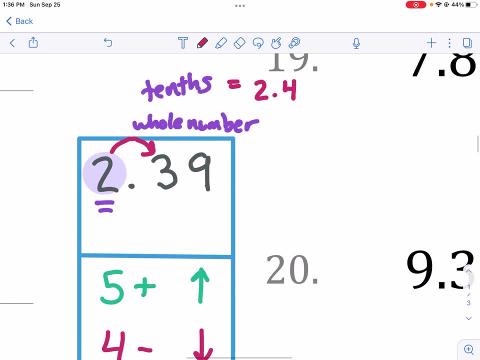 the 2.3 is. So what we're going to do is we are going to round down. So if we're going to round down, what does that mean? It means we're going to just keep the number the same. So if we're. 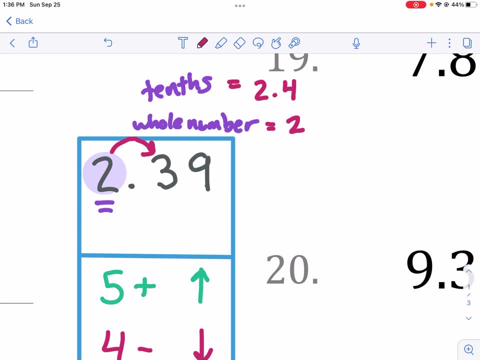 rounding down, we're just going to write two. Okay, so this two stays the same, because that three is not big enough to round it up. I've seen students make mistakes where they change it to 2.4 because or they leave it as 2.3. Because they're. 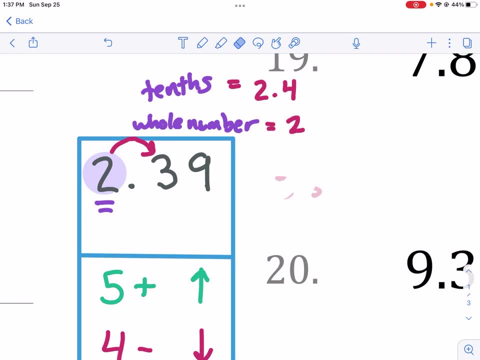 just trying to keep this whole number the same. Don't be doing that. If it's asking for a whole number, the last digit you should be writing is the whole the ones place. If it's asking for the tenths, the last digit you should be writing is the tenths place. So that's just a little helpful. 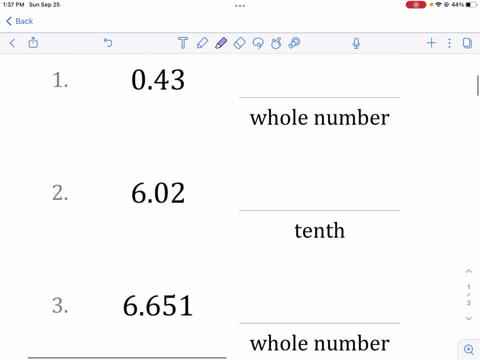 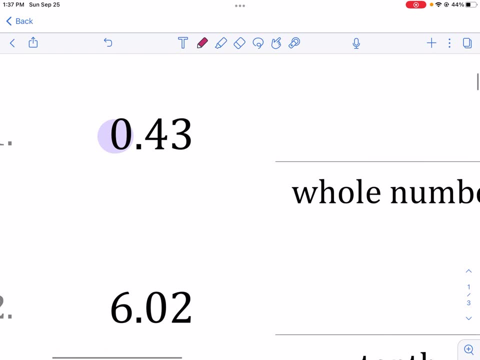 hint. Now let's go ahead and get started. So we have here: we're going to start with number one And that's a whole number. So we're going to identify the whole number And it's zero Again, we should only be writing a number that goes to the whole numbers place. We shouldn't be writing like 7.23,. 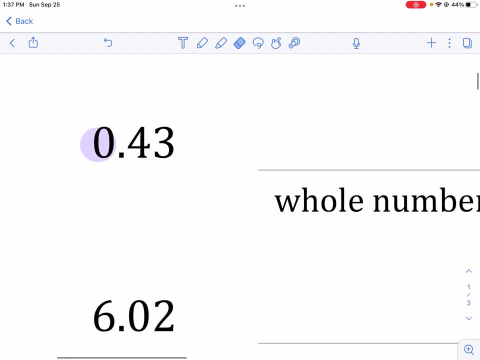 whatever, we only should be writing a whole number here for our answer. So again, we identify the whole number, place the ones place. we're going to look to the right. If it's a four or less, which this is the case, we round down. What does that mean? We just 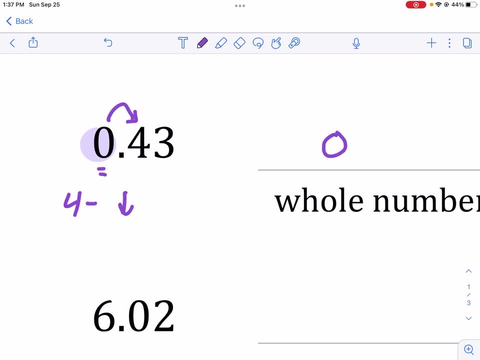 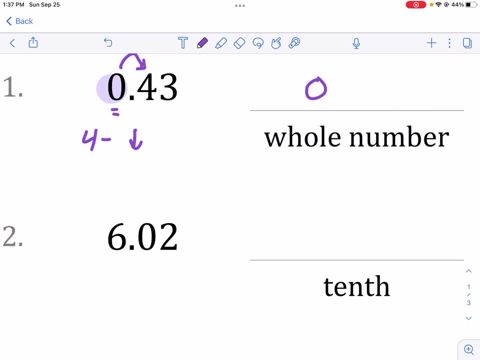 keep this number the same. So we're going to write it as zero And we're done. That's it, No more. Okay, so pretty simple. Let's do a couple more, Actually a lot more. I think we'll have time If you don't. 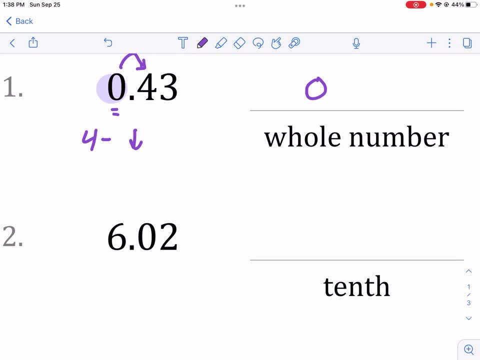 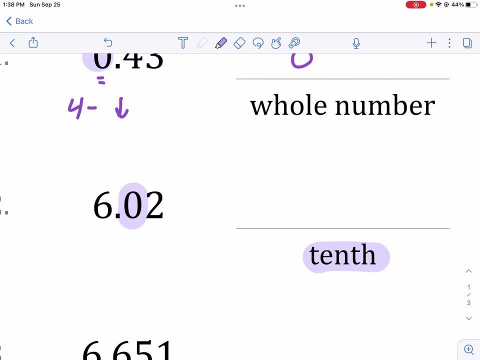 just fast forward to what you need and then get out of here. But you're welcome back anytime. I tried to get you out of here. I just want to be efficient with our time. So, the tenths place: we're going to highlight the tenths place or underline it. Okay, that's the tenths place. the 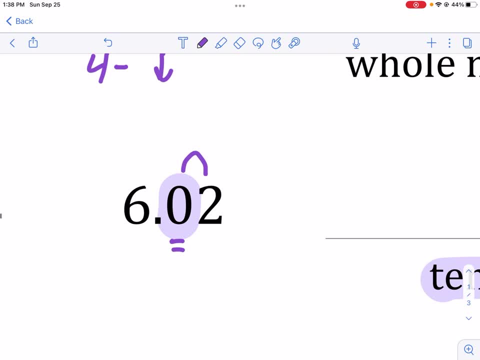 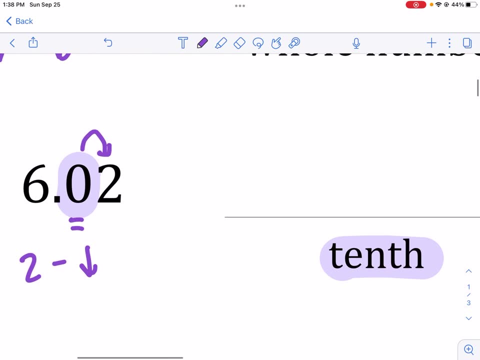 first one after the decimal place, And we're going to look to the right Again. the two is not big enough. The two is too small. So that means we're going to round down, which means we're just going to write zero for the tenths place. Okay, 6.0,. we need to write everything to the left of. 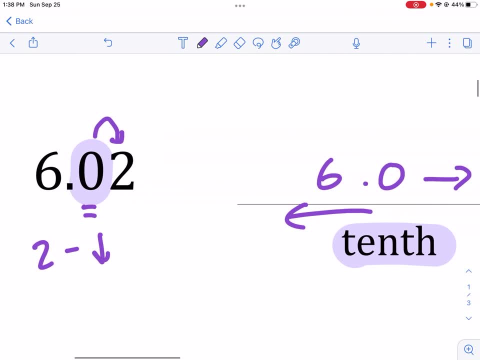 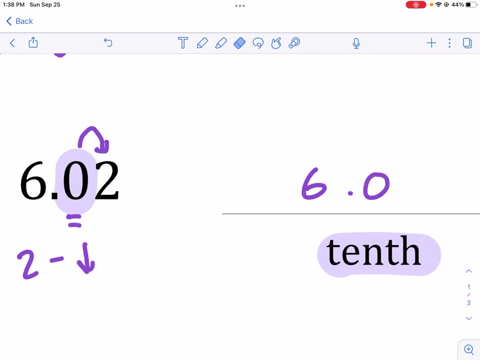 it. Also, we're going to drop anything to the right, in this case the two, and there's no other digits there, But we just leave it. we just want to write to the tenths place And 6.0 is our final. 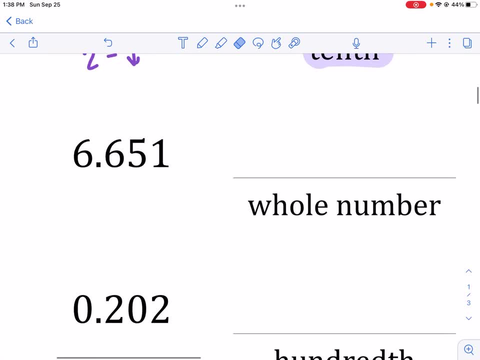 answer: Okay, 6.0.. That's rounded to nearest tenths place, whole number. Let's take a look at this one. There's the whole number, place one. we're going to look to the right And we're going to 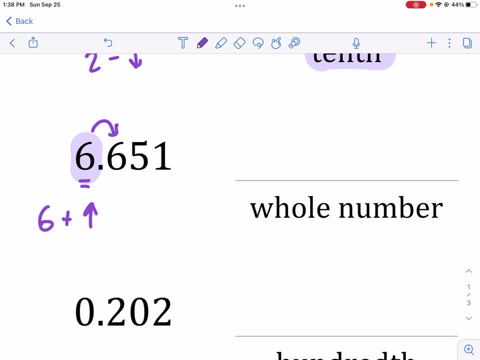 see it's a six, Remember six plus. we're going to round up Now. a common mistake, I see, is: oh, this becomes 6.7.. No, we're rounding to the whole number place. we shouldn't be writing decimals. 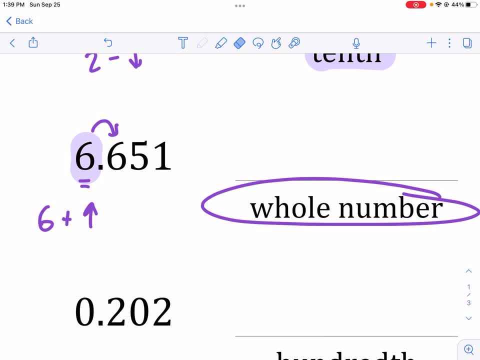 after 6.7.. So what do we round up? we round up this whole number. That means we turn it to a seven And that's it we're done. We don't write 7.0.. We don't write 7.1 or 6.7.. It's just seven. 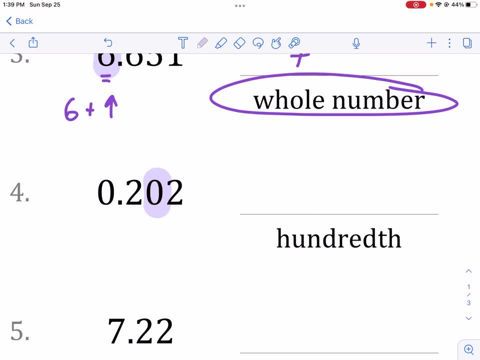 Let's go on to hundredth. This is one we haven't seen yet. Hundredth is right. there There's a hundredth place. we look to the right, it's a two. So guess what? we just keep it the same: 0.20. And we drop. 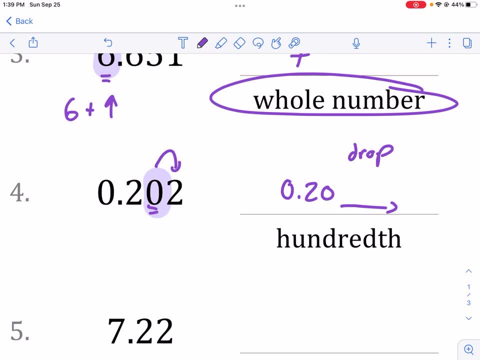 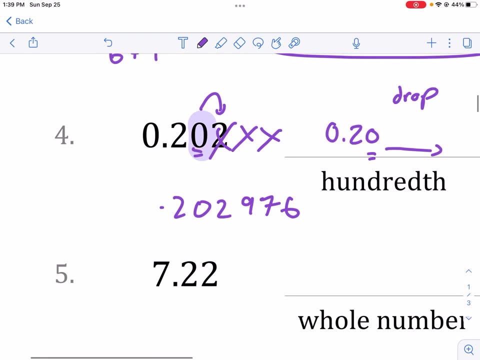 anything. rounding down essentially means we're going to drop anything to the right of our place, So our place is hundredth. we're going to drop this two here. any other numbers that we had we would also drop Okay. so if it was 0.02976, okay, really big decimal there. 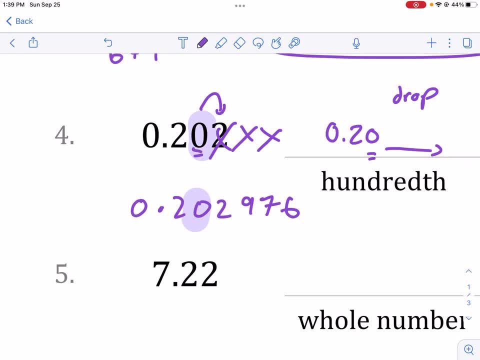 But again, if we're just running to the hundredth place, we only care about this two, We don't care about any of those other numbers. The two is not big enough, So guess what? it still would be 0.20.. 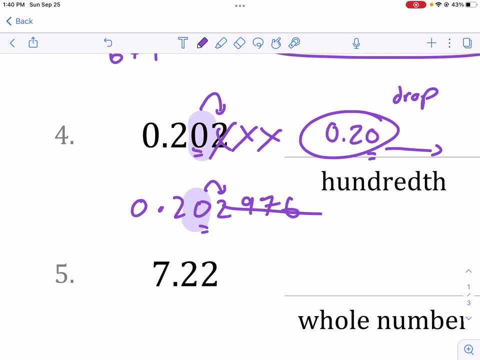 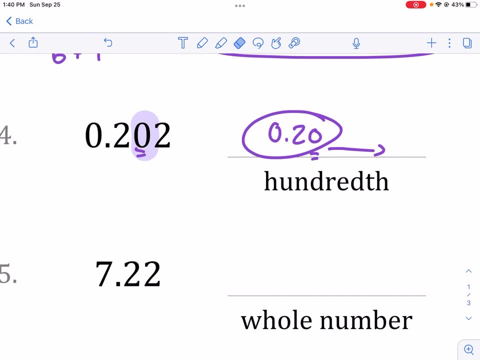 The last digit we write is the hundredth place And we drop everything else. Okay, that's essentially what rounding down is: is you're going to drop all those other things And you're going to keep that place? that's in the place value, the same. Okay, I'm going to skip ahead to some. maybe. 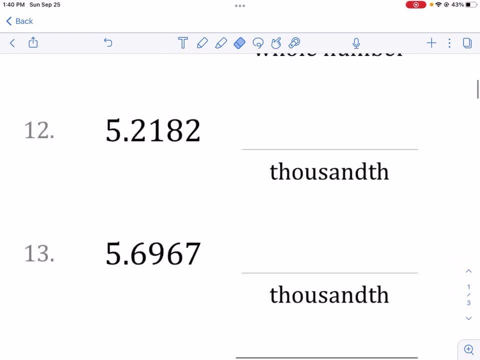 1000s or something. So let's go ahead over to the next column, And here's one. we got 1000s for number 12.. Where's that? That's the eight. we're going to look to the right here. 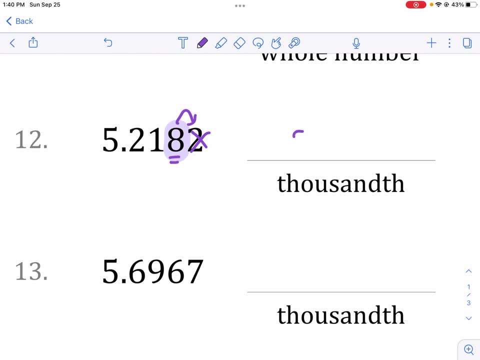 The two is not big enough. So we're going to keep this the same And we're going to drop that to 5.218. is our answer there? 1000s for this one. Let me get rid of the highlighter. Here's the. 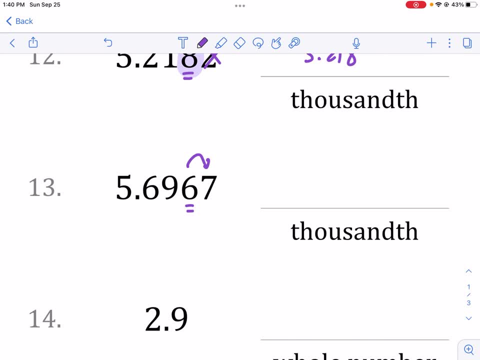 1000s. We look to the right, we see it's a seven. that means we're going to round up. Okay, so we're going to write 5.69.. The number that we underline is the one that we round up or keep the same for. 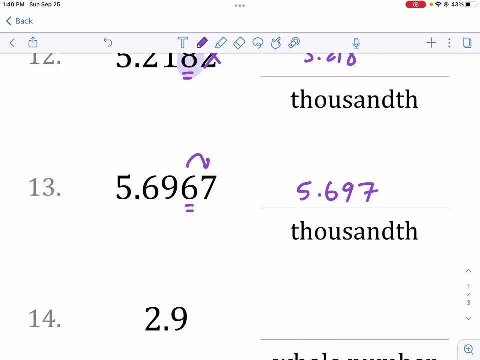 rounding down Seven: 5.696.. Seven would be our answer there. Okay, we don't care about that seven, you don't keep it there, You just get rid of it. I want to see one that we round. Aha, this is what I wanted, to take a look. 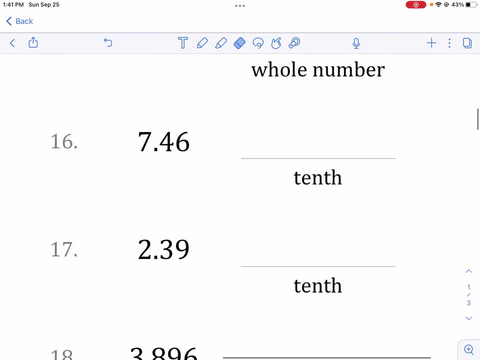 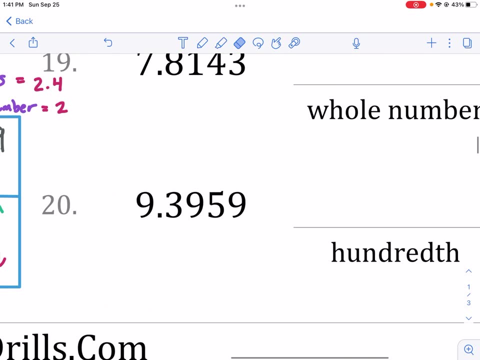 at. Oh no, not this one, I want one where the place we're trying to round is, in fact, a nine. Okay, great, So number 20.. This is the last one I want to do. We're going to identify our place. 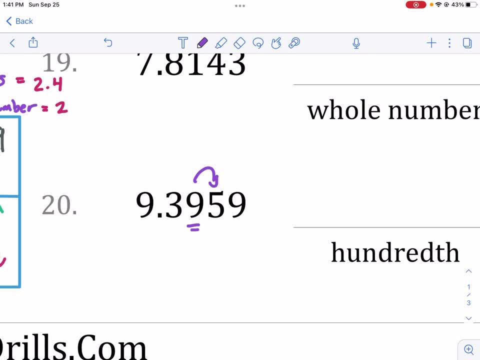 Okay, I said I was going to underline: Here we go, There's our place, We look to the right of our place. So five, that means we need to round up, So we have 9.3.. What's above? nine: we don't write a 10.. 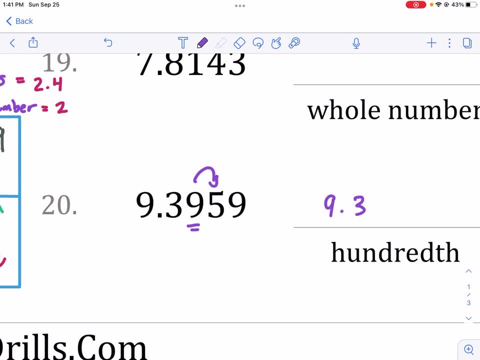 So what we do if this is a nine is it's like a double round. Okay, this five tells the nine to round up. it has nowhere to go, So we need to essentially bump up this three instead. Think of it this way: Okay, If we were to round this down, it would be 9.39.. But if we want to round it up, 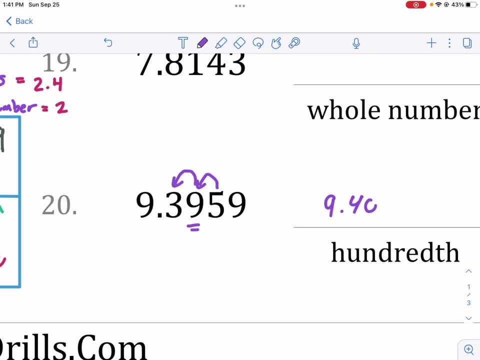 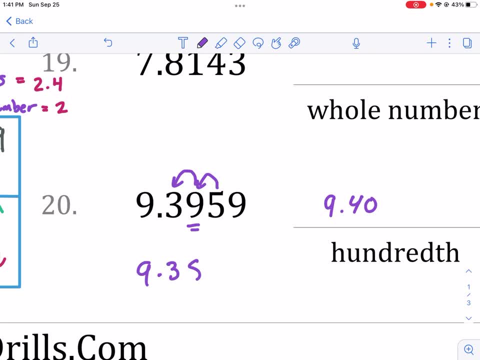 40. So normally again, if this were 9.385, and we round to the nearest hundredth, this would change to 9.39.. But since it's already 9.39, with that, five nine there. okay, we are going to bump. 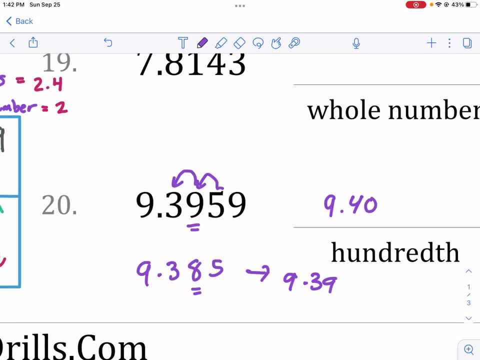 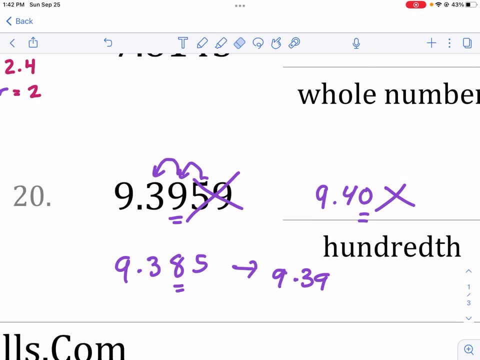 up this nine to become a 10,, which increases that three, So 9.40.. And again, the last digit we should write is that hundredth- We don't care about those other digits past it anymore- And it stays at 9.40.. That's all the time we have for today. Thank you for watching this.